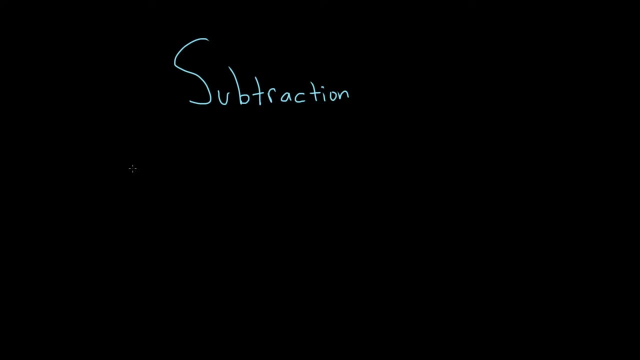 Hi everyone, in this video we're going to do some examples of subtraction. Let's just start right away. Let's say we have 27 minus 6. So what we do in a situation like this is you write down the 27 and then we line it up with the 6. So we keep all of the place values the same. So the 6 goes right under the 7 because these are both in the ones place. Then you draw a line and you put like a minus sign here like this. That means we're going to subtract. Then you just subtract you know place value from place value. So 7 minus 6 is 1 and there's nothing here. So you just bring down the 2. So 21. So that's it. This was a purposely easy example. What if it was a little bit harder? What if it was 27 minus 16? So in this case you would write down the 27 and just like before you would line it up. So you write down the 16 right below it like this. You draw a line and then you have a minus sign. And again you just subtract the same way. 7 minus 6 is 1. 2 minus 1 is 1. So 11 is the answer. So still pretty easy right? A little bit a little bit harder but not too much harder right? You're just subtracting each column. Sometimes though certain things happen which makes it more difficult. For example, if you have a column and you have a column and you have a column , for example say we have 885 like a big step up to 27. Minus 57 just like before we line them up so 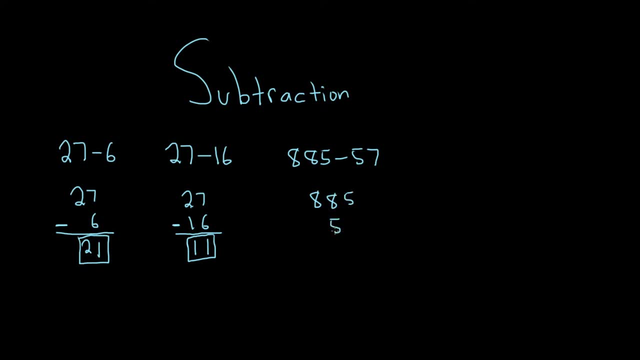 885 and then you put the 57. Here we draw our line and then you subtract. Well there's an issue here right? You have 5 minus 7 so this number up top needs to be bigger. So what you do is you borrow 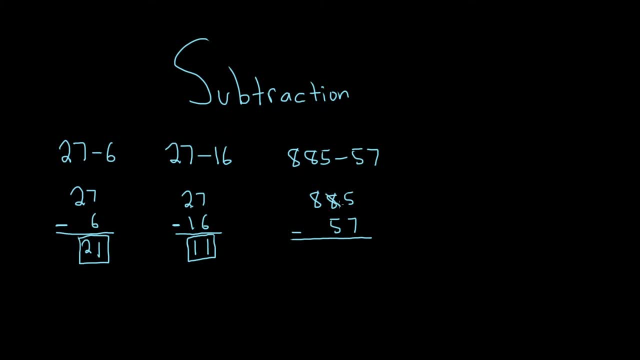 is you borrow one from here. So you put a line through it, and then you subtract one from it. So you borrow a 10. So you make this a 7, and then you make this a 15. 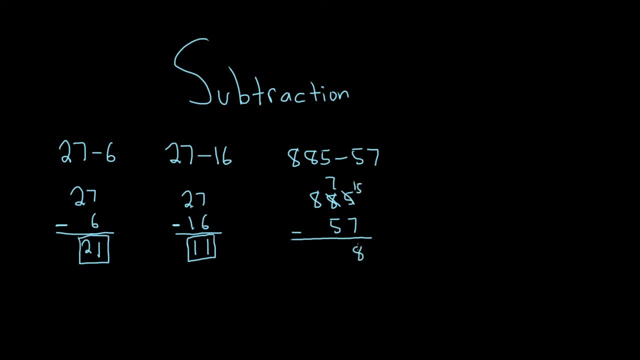 So 15 minus 7 is 8. 7 minus 5 is 2, and then you bring down the 8 again. It's a little bit sneaky. Let me go over that again. 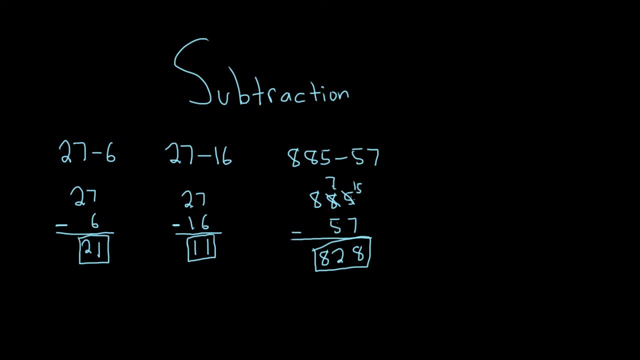 So that was a big step up in difficulty. So because the 5 is smaller than the 7, you can't do the subtraction using this method. So what you do is you borrow one of the 10s from the 10s place. So you cross out the 8, and you subtract one, and you put a 7. And then you say, OK, now I have a 15 here because I borrowed a 10. So 15 minus 7 is 8. And then when you go to the next step here, this is going to be 7 minus 5, which is 2, and then you bring down the 8. 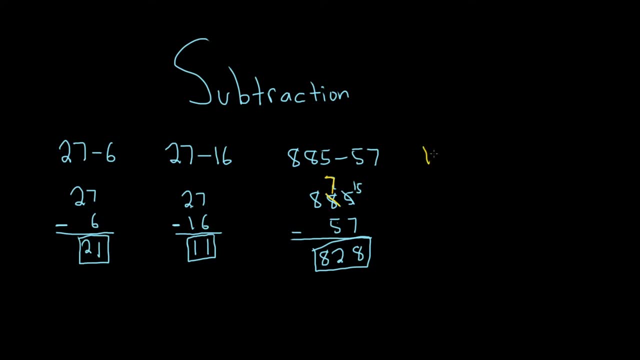 Let's do another one. Let's say we have 100. And 61 minus, I don't know, how about 22? 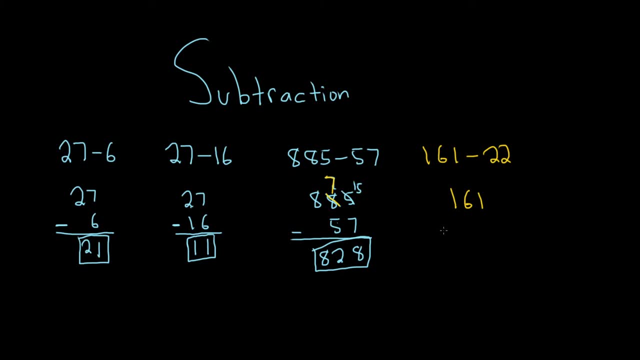 So same thing. We line them up. 161 minus 22. 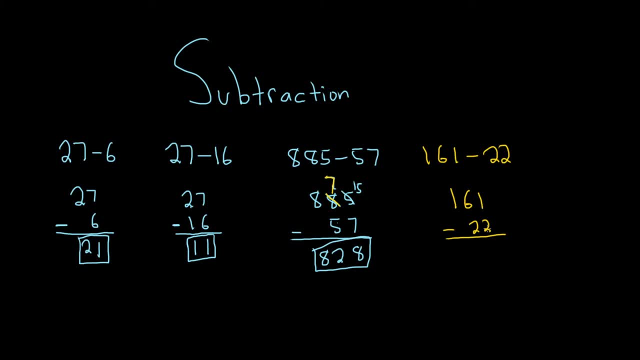 So same thing. See, 1 is smaller than the 2. So we can't subtract them. 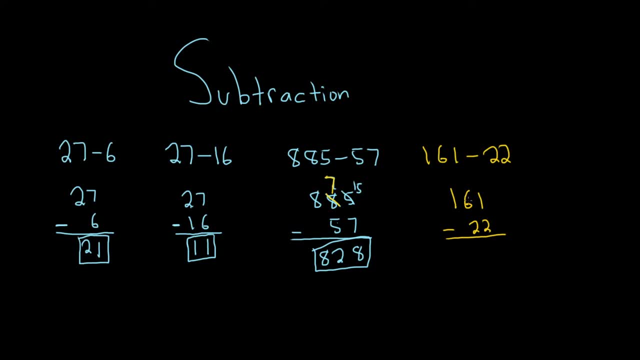 So what you do is you come over here to the next digit, to the next place value, and you borrow one from here. You make this a 5, and then you make this an 11. You just add 10 to it every time. It's like over here, the 5 became 15 because we added 10. Here, the 1 becomes 11 because we added 10. And then you subtract. 11 minus 2 is 9. And then 5 minus 2 is 3. 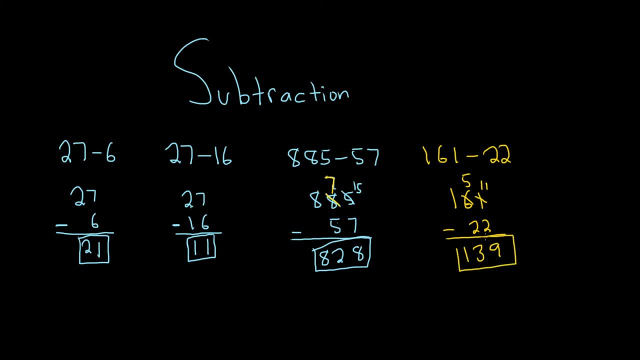 And then you bring down the 1, and that's 139. So a little bit harder examples. 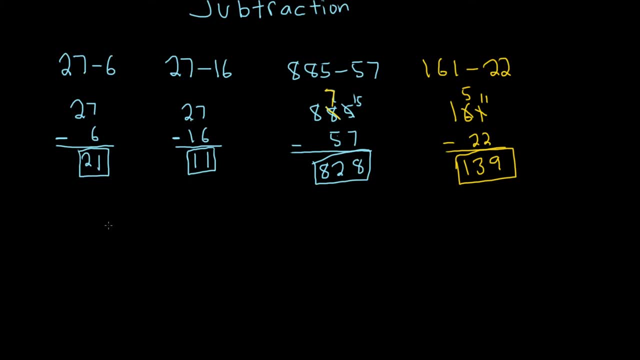 Let's do another one. Let's say we had something even harder. Let's say we have 903, it's about as hard as it gets, minus 256. 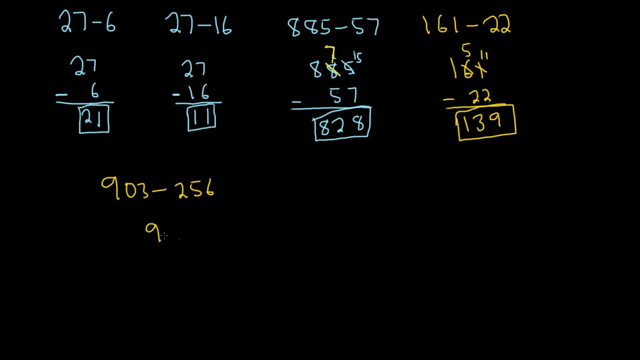 So just like before, we line them up. We write down the 903, and then here's the 256. And then we draw our line, and we put our minus sign here. So already there's a problem. 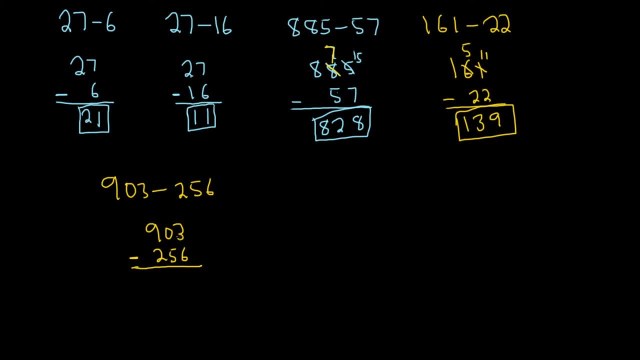 You see, the 3 is smaller. So we want this to become a 13. You say, okay, so I want to borrow one from here. But you can't borrow from 0. It doesn't work. So what do you do?